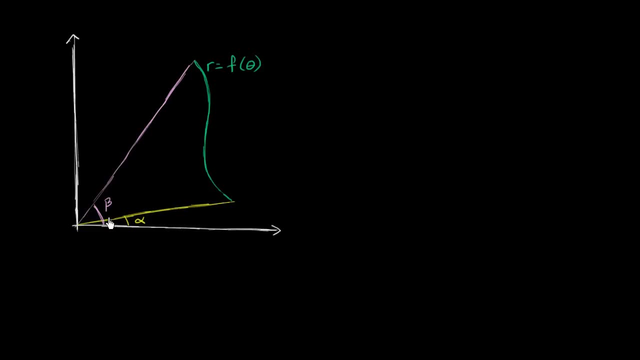 and we were able to find the area. But now let's move on to polar coordinates, And polar coordinates- I won't say we're finding the area under a curve, but really in this example right over here we have a part of the graph- of r is equal to f of theta. 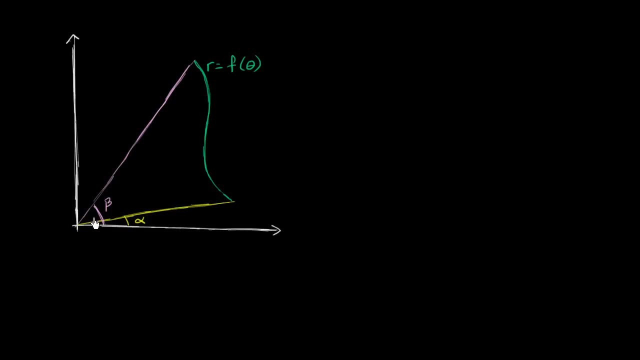 and we've graphed it between: theta is equal to alpha and theta is equal to beta, And what I wanna do in this video is come up with a general expression for this area in blue, this area that is bounded, I guess you could say. 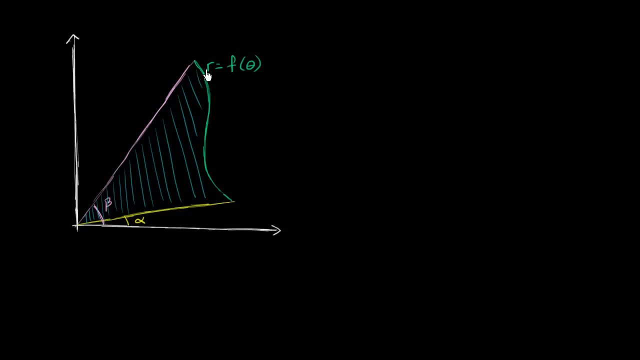 by those angles and the graph of r is equal to, r is equal to f of theta, And I want you to come up, or at least attempt to come up with an expression on your own. but I'll give you a little bit of a hint here. 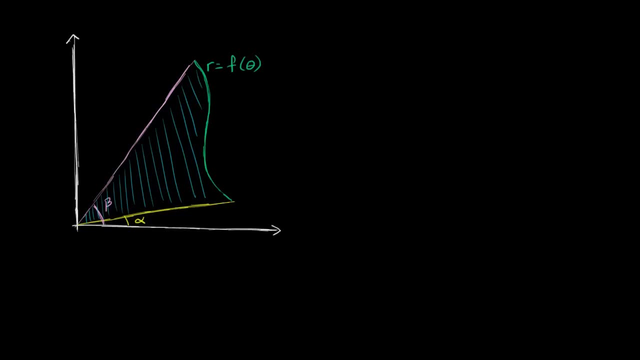 When we did it in rectangular coordinates, we divided things into rectangles. Over here rectangles don't seem as obvious because they're all kind of coming to this point. But what if we could divide things into? if we could divide things into sector? 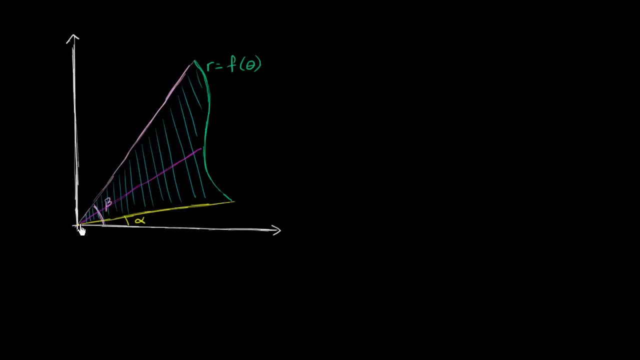 I guess we could say: little pie pieces. Someone's doing some serious drilling downstairs. I don't know if it's picking up on the microphone, but anyway I will continue. So what would happen if we could divide this into a whole series of kind of 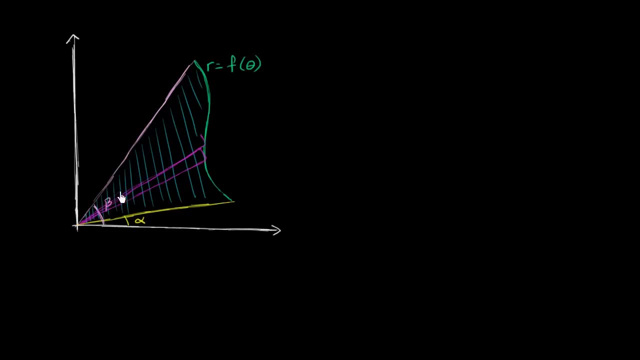 pie pieces, If we could divide it into a whole series of pie pieces And then take the limit as if we had an infinite number, an infinite number of pie pieces. So we want to find the area of each of these pie pieces and then take the limit as the pie pieces. 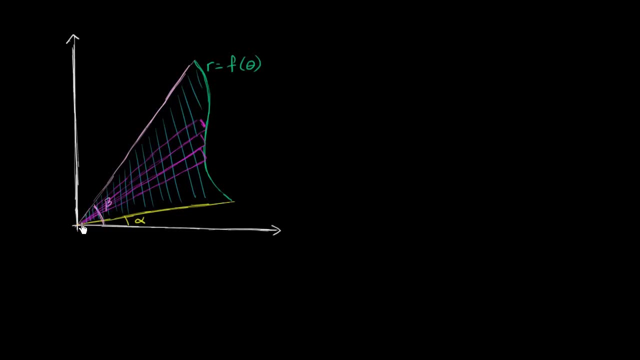 I guess you could say: become infinitely thin, and we have an infinite, and we have an infinite number of them. And I'll give you one more hint. I'll give you one more hint for thinking about the area of these pie. I guess you could say pie. 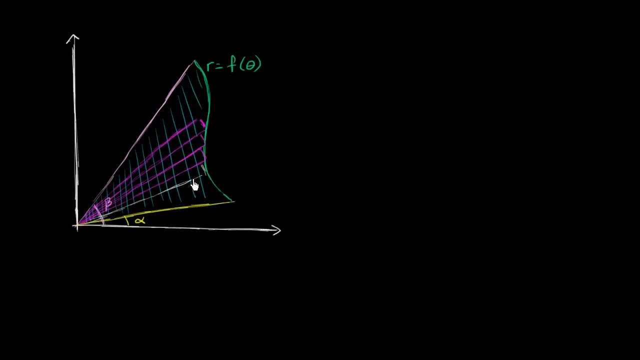 the area of these pie wedges. I'll give you another hint. So if I have a circle under my best attempt at a circle, luckily the plumbing or whatever is going on downstairs has stopped for now, allowing me to focus more on the calculus, which is obviously more important. 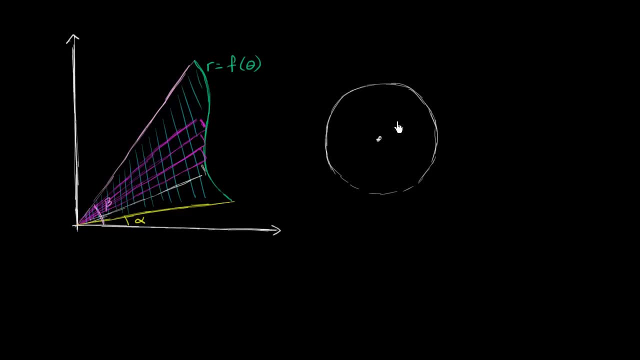 All right. so if I have a circle, that's my best attempt at a circle, and it's of radius r, it's of radius r and let's say, let me draw a sector of this circle. It's a sector of a circle. 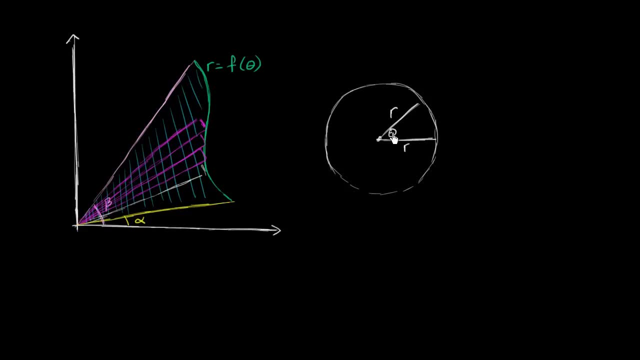 So that's obviously r as well. And if this angle right here is theta, what is going to be the area, what is going to be the area of this sector right over here? So that's my hint for you: Think about what this area is going to be. 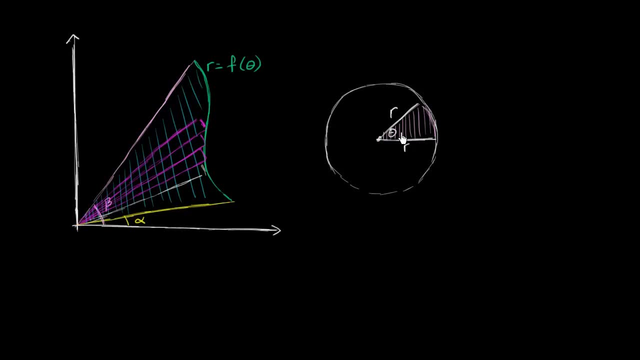 and we're assuming theta is in radians. Think about what this area is going to be and then see if you can extend that to what we're trying to do here to figure out a somehow. I'm giving you a hint again- using integration. 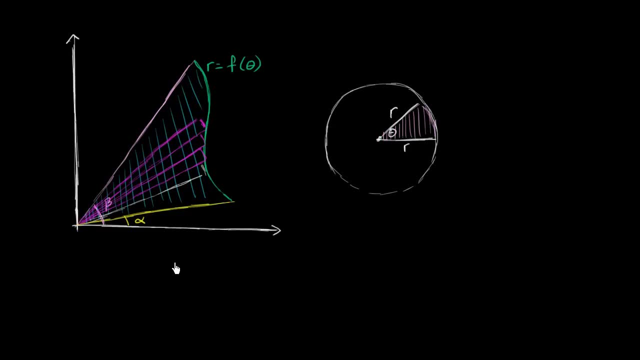 finding an expression for this area. So I'm assuming you've had a go at it. So first let's think about this: So what's the area of the entire circle? Well, we already know that That's going to be pi r squared. 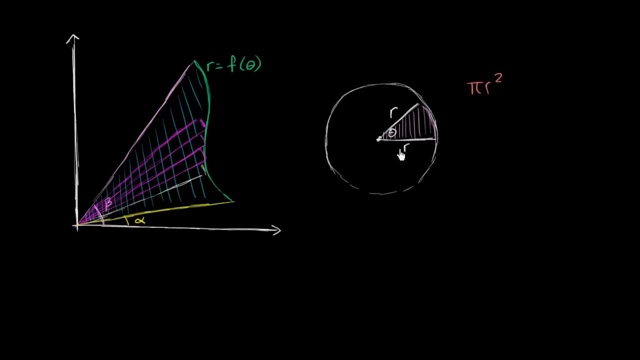 formula for the area of a circle. And then what's going to be the area of this? Well, it's going to be a fraction of the circle. If this is pi sorry, if this is theta where, if we went two pi radians. 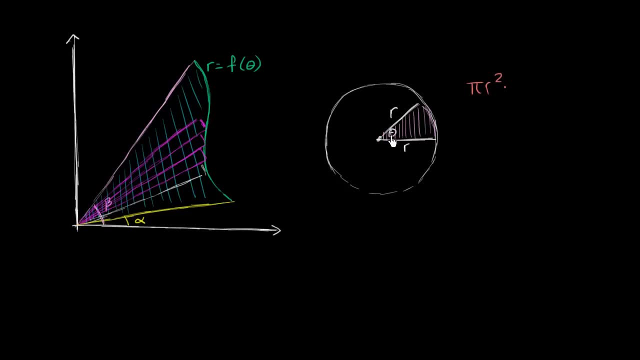 that would be the whole circle. So this is going to be pi. sorry, this is going to be theta over two pi of the circle. So times theta over two pi, times theta over two pi, would be the area of this sector right over here. 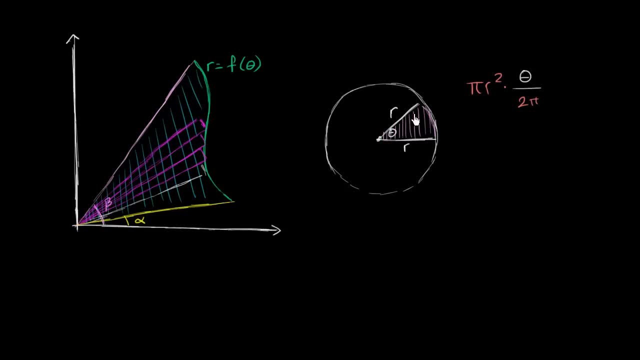 area of the whole circle times the proportion of the circle that we've kind of, we have defined, or that the sector is made up of. And so this would give us this would give us the pi's cancel out. it would give us 1 1⁄2 r squared times theta. 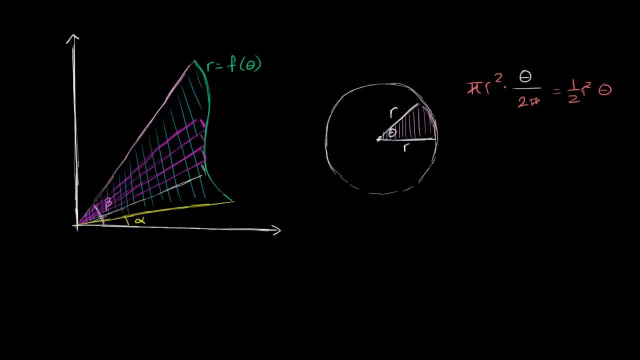 Now, what happens if, instead of theta, so let's look at each of these over here, So each of these things that I've drawn, So let's focus just on one of these, one of these wedges. I will highlight it in orange. 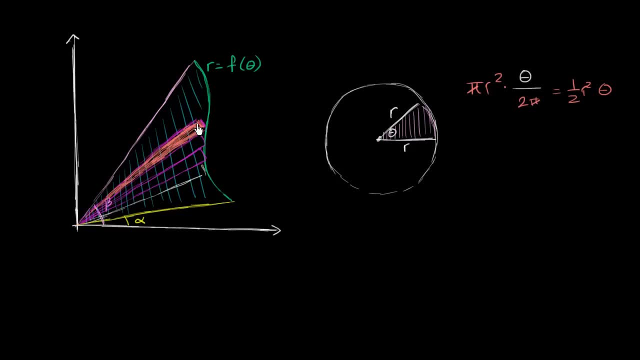 I'll highlight it in orange. So instead of the angle being theta- let's just assume it's a really, really, really small angle- We'll use a differential, although this is a little bit of loosey-goosey mathematics, But the important here is to give you 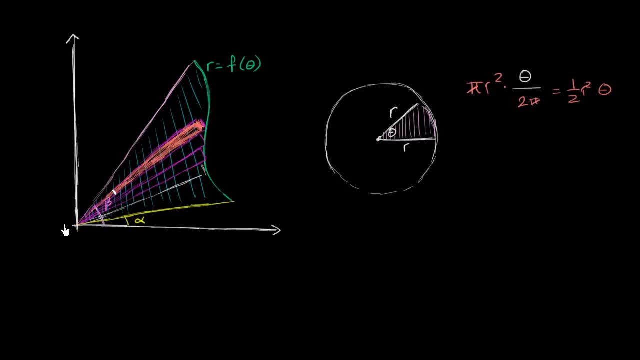 the conceptual understanding, I could call it a delta theta and then eventually take the limit as our delta thetas approach zero. But I'm just gonna, just for conceptual purposes, assume we have a infinitely small or super small change in theta, So let's call that d theta.